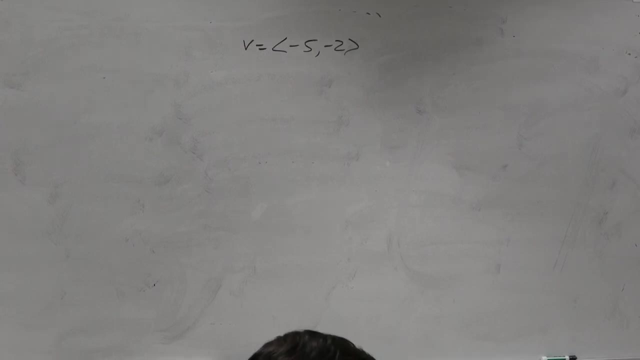 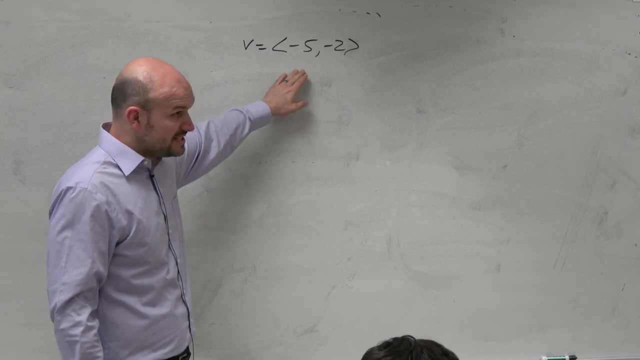 Not only is it not a good best use of your time all the time, but sometimes, guys, you need to also understand the context of what you're doing. The calculator's not going to save you. For instance, this example. So we can find the magnitude using the formula that: 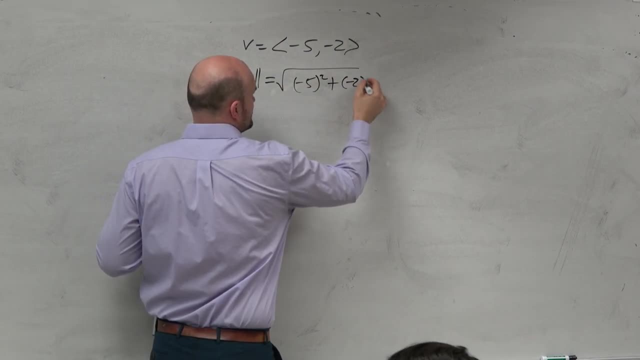 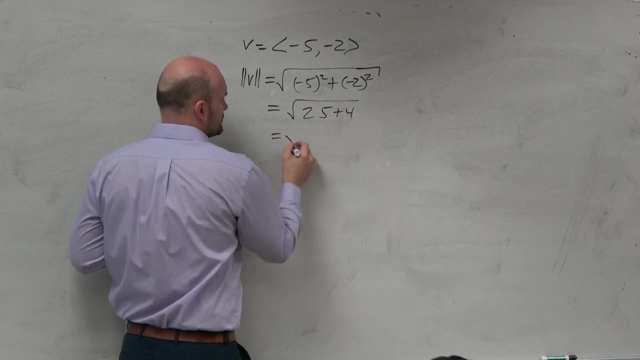 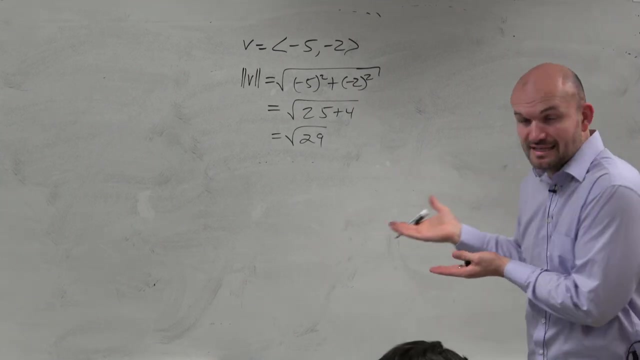 is just the first component squared plus the second component squared. So therefore, in this case, we're going to have 25 plus 4, which equals the square root of 29.. I got it. Now let's go to the direction. I don't recognize anything special about this. Agreed. 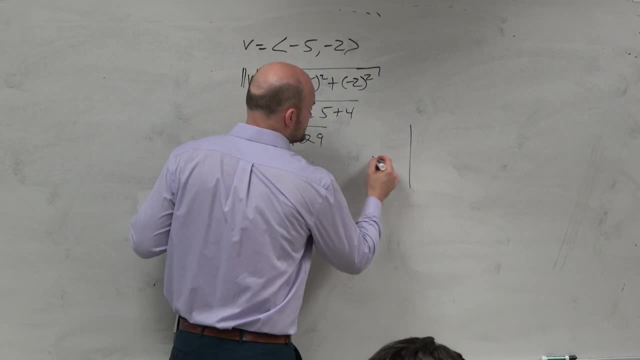 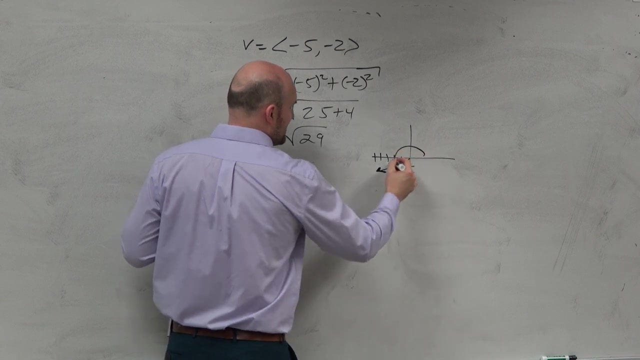 But I will say though, if I was to graph this vector- 1,, 2,, 3,, 4,, 5,, 1, 2, then my vector is going to look somewhere here. So if I'm trying to find this angle here, I'm looking. 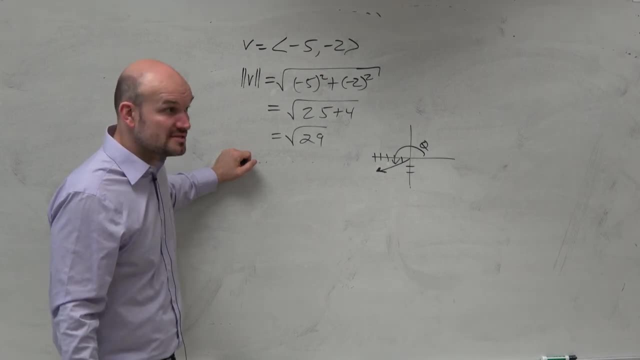 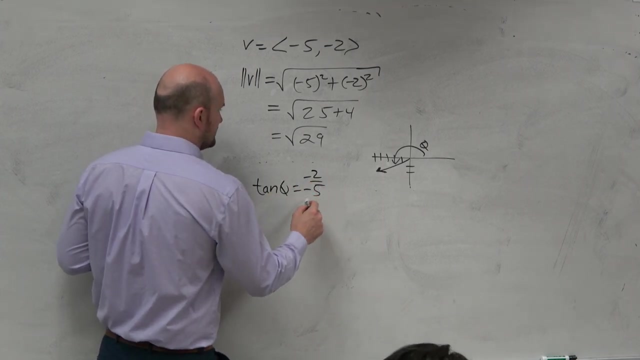 for that Agreed. That's the angle I'm looking for- Standard form. So I'm going to follow the formula. Tangent of theta equals negative 2 over negative 5.. Right V2 over V1.. Theta equals tangent. 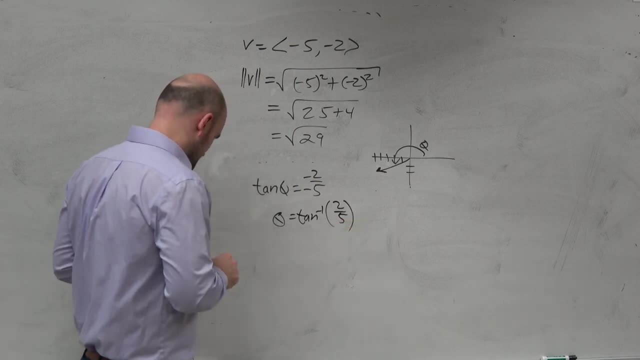 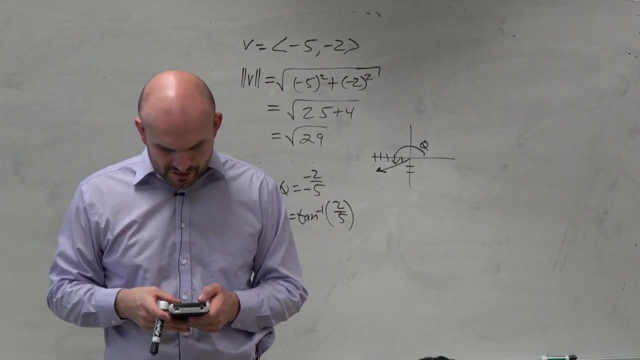 inverse. We can just do a positive of 2 fifths. So I go ahead and grab my calculator. I say, all right, Tangent inverse of 2 divided by 5. 21.8.. That does not look like the right. 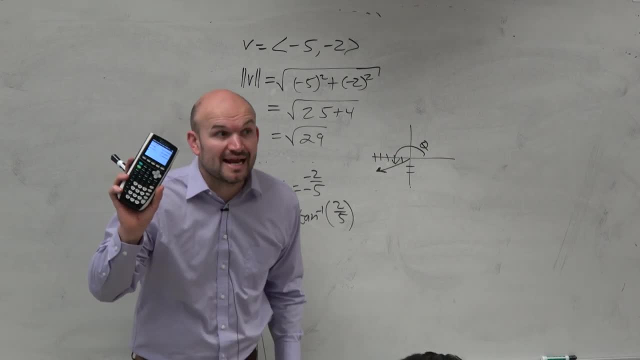 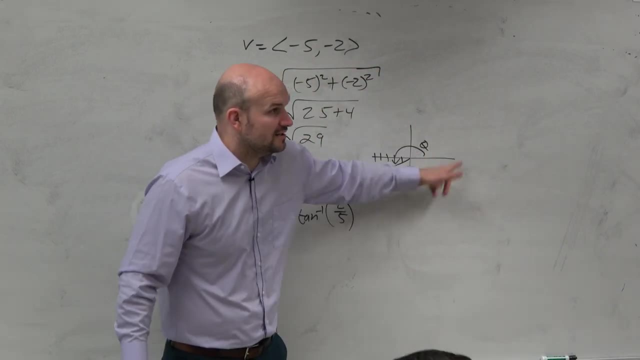 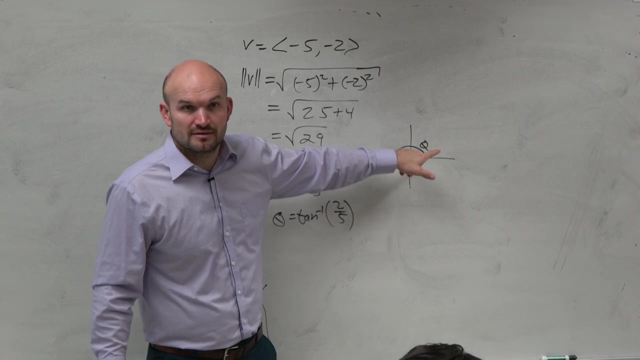 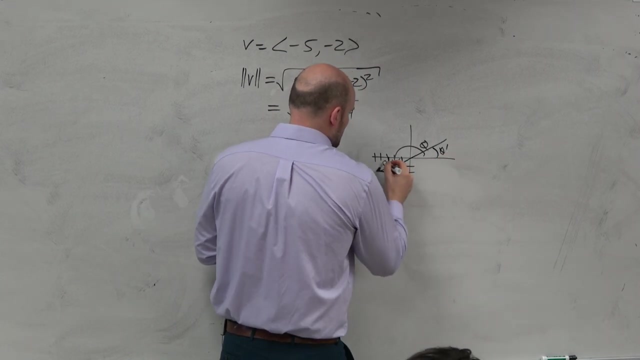 angle. Yes, it does. It does Now remember we're going to have two angles here. The angle that's 21.8.. What does 21.8 look like? I say it looks like this right here, See 21.8.. 21.8., 21.8.. Right. So the calculator gave me the answer. It's not going. to save me. I need to understand what the calculator has given me. Remember, guys, tangent inverse is only restricted from here to here. It's not going to give you this angle, Agreed, It's only giving you this. So what has it actually given me? It's given me this angle, this reference. angle. It's giving me the reference angle, So that means that's 21.8.. That's 21.8.. So if I need to find the angle from there to there, that's 21.8.. So what's going to happen here Now? because you didn't.